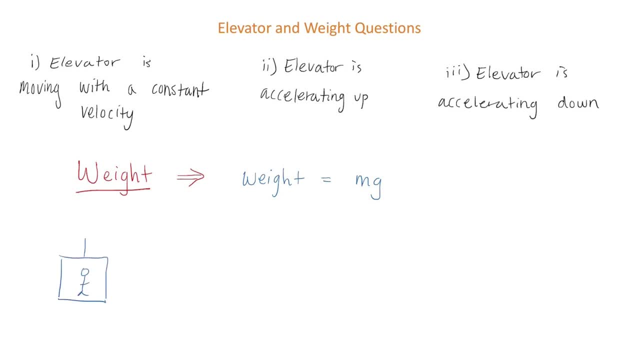 pushing down on it. But why then, would a person in an elevator that's accelerating up feel heavier, Or a person who's in an elevator that's accelerating down feel lighter? Well, the answer is, the person's actual weight is not changing, but their apparent weight is, And 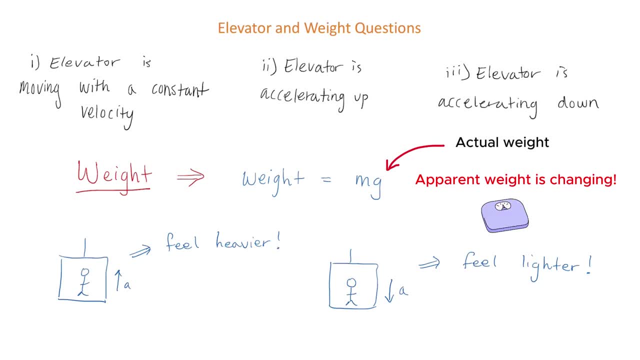 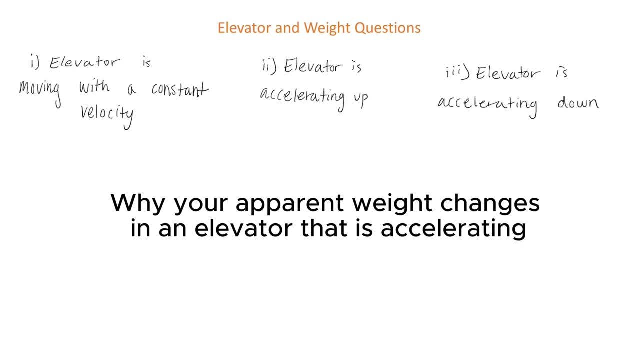 your apparent weight is the weight that would be measured on a scale, whereas your actual weight is the force of gravity that's pushing down on you. So in this video, we are going to learn why your apparent weight changes if you are in an elevator that is accelerating down. 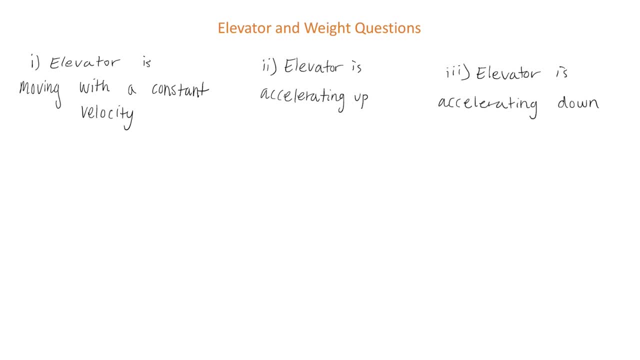 We are going to look at three situations. The first is an elevator that is moving with a constant velocity. The second is an elevator that's accelerating up. And the third is an elevator that's accelerating down, And we are going to assume that there's a 70 kilogram person standing in an elevator. 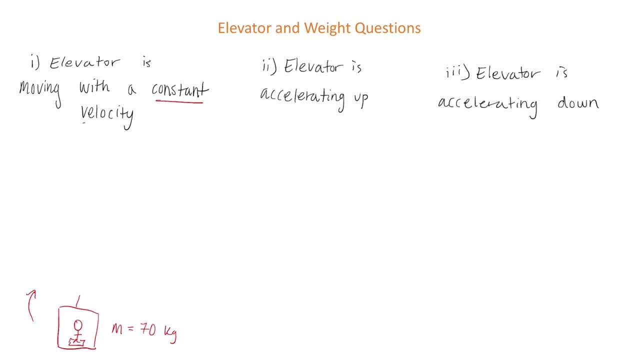 So in the first situation we have an elevator that is moving with a constant velocity. When you hear constant velocity, you should recognize that the acceleration is equal to zero, which means the net force acting on this elevator and the person inside it is zero. So if we draw a free body diagram, 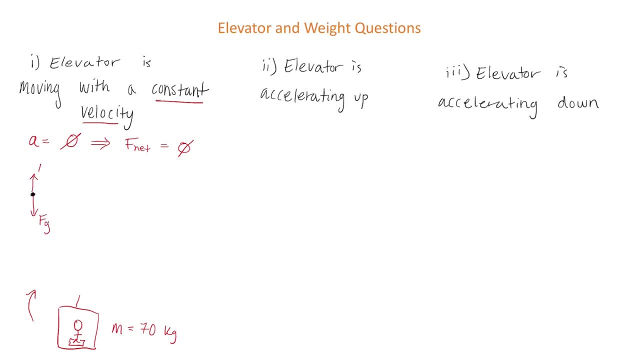 for the person, we would have the force of gravity and the normal force, And now we can write an f? net equation which would be the sum of all the forces acting on this person. So we have the normal force minus the force of gravity. We can replace f? net with zero. 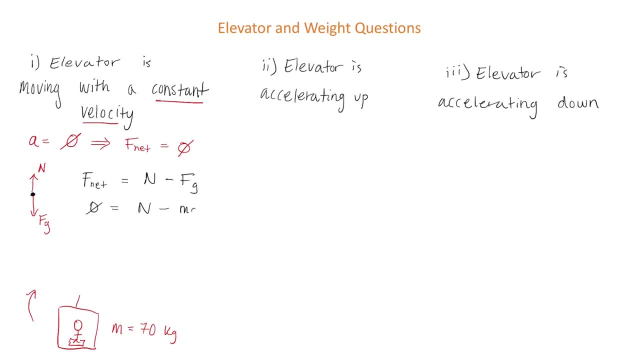 because there's no net force acting on this person And we can replace the force of gravity with mg. Then I can rearrange this equation and solve for the normal force And we see that the normal force is equal to mg. And now the reason I rearranged this equation: to solve for the normal force. 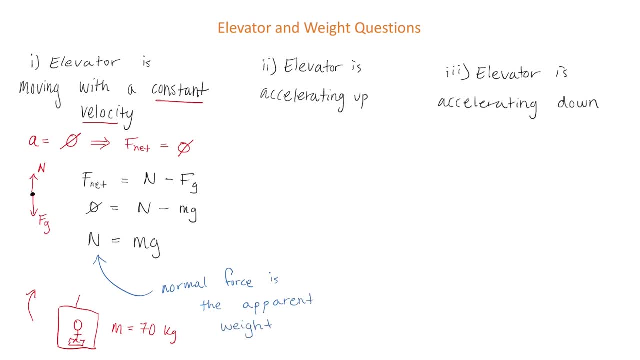 is because the normal force represents the person's apparent weight. So I can just plug in my values and what we find is that the apparent weight of this person is 686 newtons. But now let's look at the case where the elevator is accelerating. 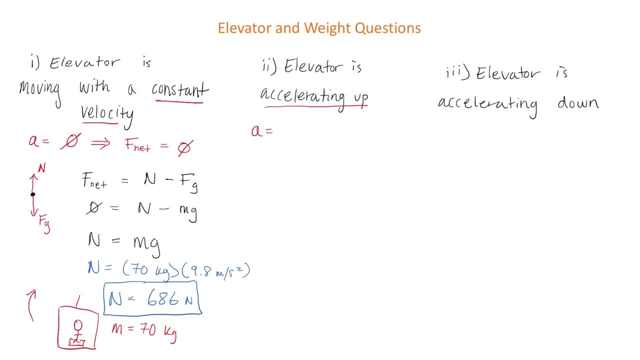 up And we are going to assume the acceleration is equal to two meters per second squared. So again I will draw a free body diagram with the force of gravity and the normal force. But because the object is accelerating up, I know the net force should be pointed up. And now I'll make an f? net. 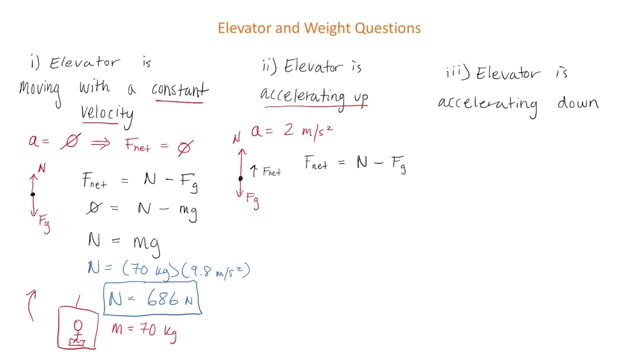 which represents the normal force minus the force of gravity. and this time I have to replace f net with ma, because the elevator is accelerating, But let's do this again. So I'll also replace the force of gravity with mg and then I will rearrange and isolate for the normal force. 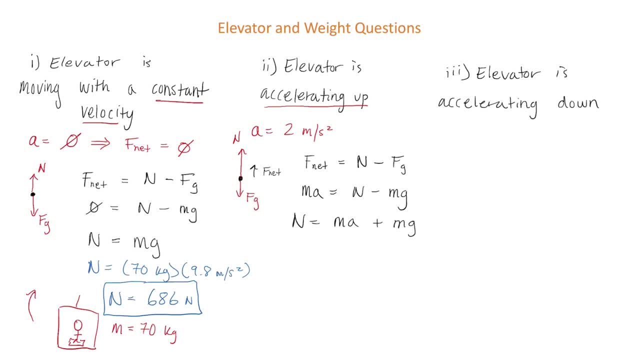 And now- I hope you can see this- now that the normal force, which represents the apparent weight of the person in the elevator, has an additional term, And so when I plug that嘱, plug in all my values, we can see that the normal force is 826 newtons, which is larger than the 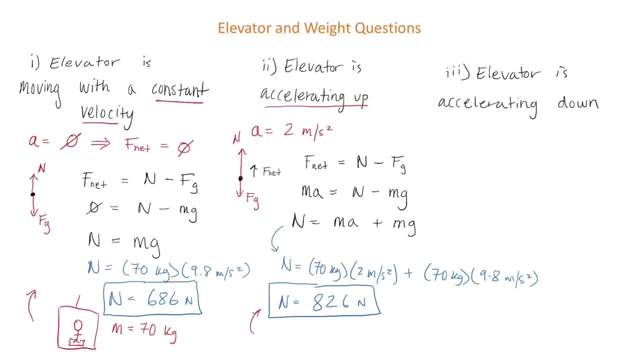 normal force when the elevator was moving with a constant velocity. And since the normal force represents a person's apparent weight, because it's larger, the person will feel heavier as they're accelerating up. Now let's look at the case where the elevator is accelerating down. 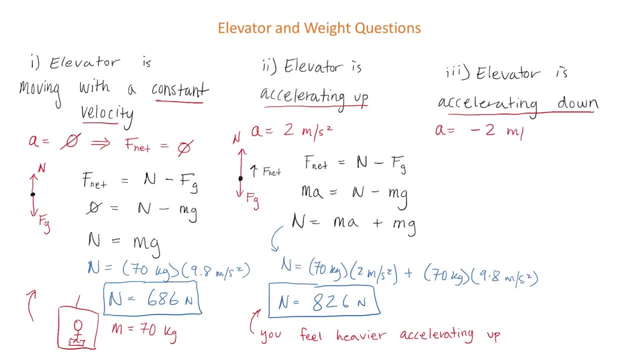 And in this case we'll assume the acceleration is equal to negative, two meters per second. squared. It's negative because the elevator is accelerating down, And so I will draw my free body diagram, which is just the force of gravity and the normal force, And the net force is going to be pointed. 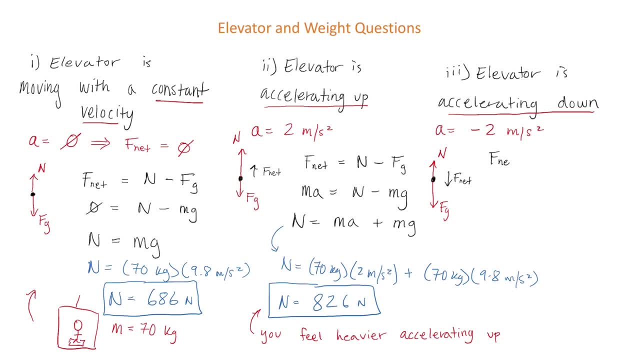 down, Then I will write my net force equation. So we have: F net is equal to the normal force minus the force of gravity. I replace F net with MA. I replace the force of gravity with mg. I rearrange and isolate for the normal. 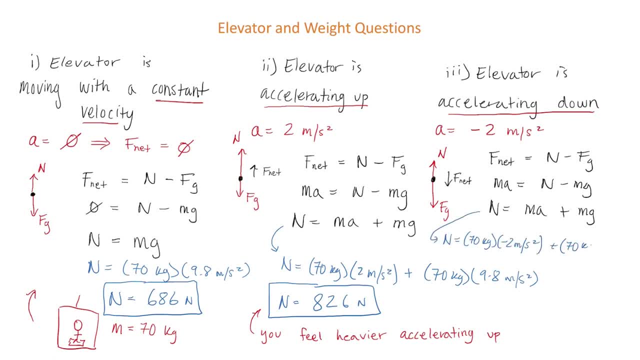 force. and again I will plug in my values and what we find is that the normal force is equal to 546 newtons. and now notice: this normal force is smaller than when the elevator was moving with a constant velocity and then when the elevator was accelerating up. That means the person's apparent weight is smaller. 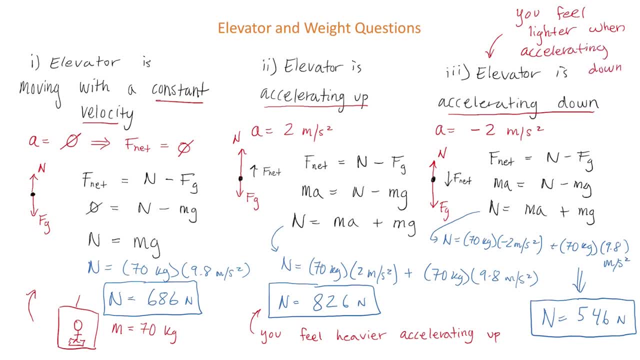 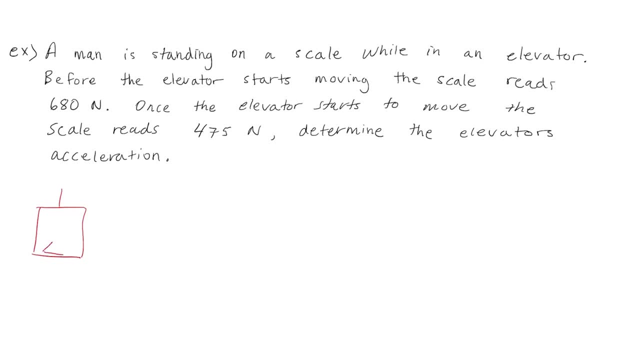 and that explains why you would feel lighter when you're accelerating down in an elevator. Now let's do an example to practice what we learn. We are told that there is a man standing on a scale while in an elevator. Before the elevator starts moving, the scale reads 680 newtons, but once the elevator starts, 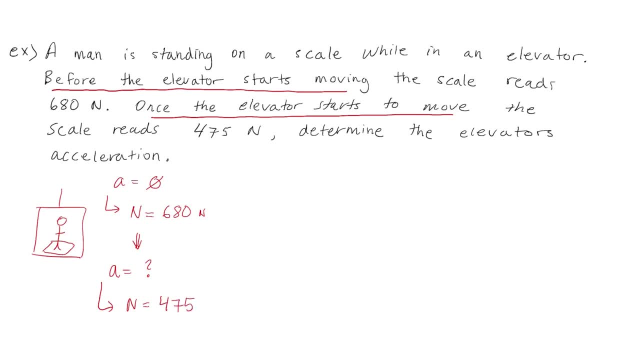 moving. the scale reads 475 newtons and we want to determine the elevators acceleration First. let's only consider when the elevator is not moving. If we draw a free body diagram, we know we have the force of gravity and the normal force and we 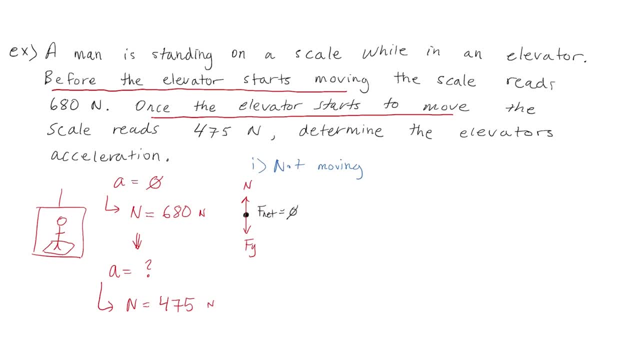 know the net force is equal to 0 because the elevator is not moving. Then we make our F net equation, which is just the normal force minus the force of gravity, and we replace F? net with zero, and then we replace the force of gravity with mg. 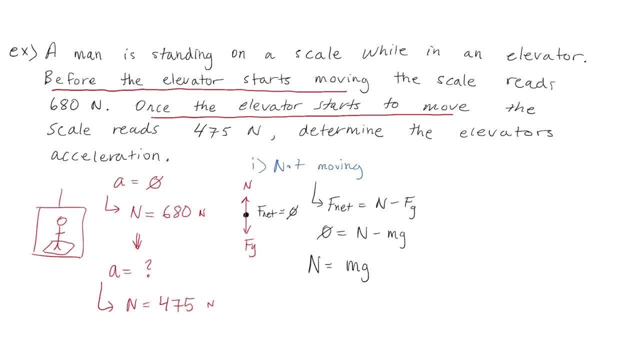 and then I will just rearrange and isolate for the normal force. And so we have the normal force, we have the acceleration due to gravity, but what's missing is the person's mass. So we can rearrange this equation and solve for the person's mass, and what we find is the man's mass is 69.4 kilograms. Now, 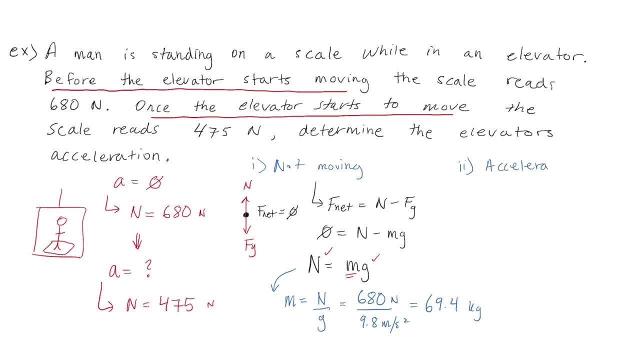 that we know the person's mass. let's look at what happens when the elevator starts to accelerate. If we draw our free body diagram, we have the force of gravity and the normal force and I know the net force will be pointed down and that's because the person's apparent weight decreased. 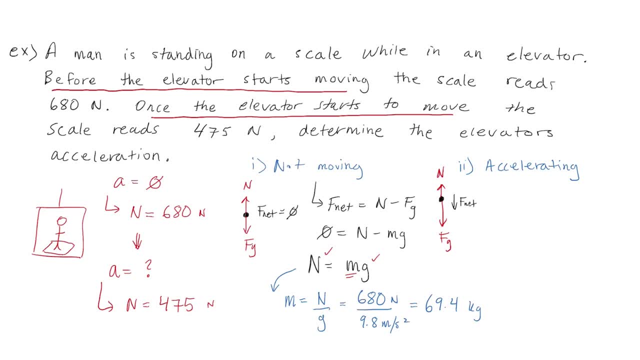 once the elevator started accelerating- and we know that happens when the elevator is accelerating down- Then I will write my F net equation, which would be the normal force minus the force of gravity. I replace F net with ma and I replace the force of gravity with mg. but then I have to remind myself that we are 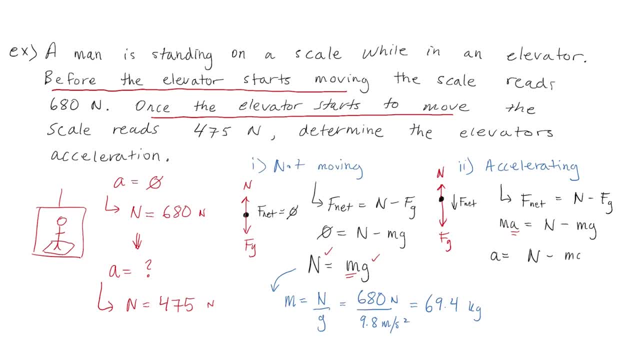 solving for the elevator's mass acceleration. so I will rearrange and isolate for the acceleration. Then all I have to do is plug in my values and what we find is the object's acceleration is equal to about negative 2.96 meters per second squared, and it makes sense that.